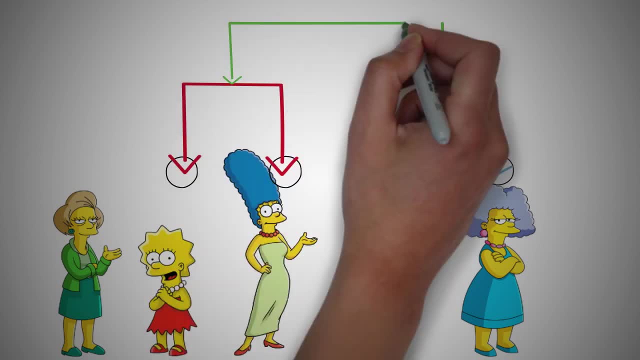 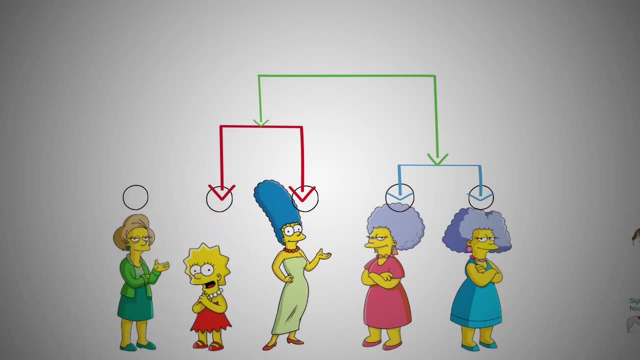 We merge the Lisa and Marge cluster with the twins cluster, mainly because they are closer than they are to Edna Flounders. So now we join them into one cluster And finally we join our mega cluster with Edna And you can see how long the process takes. So we can see how long the process takes. 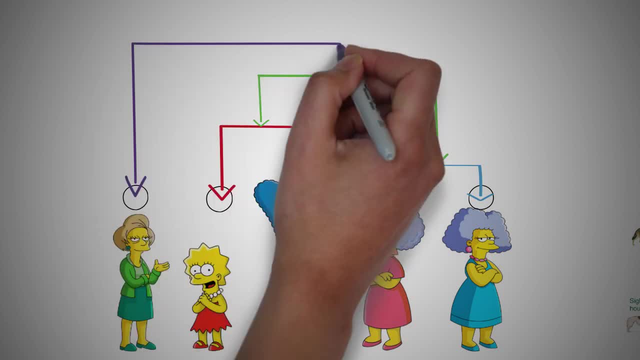 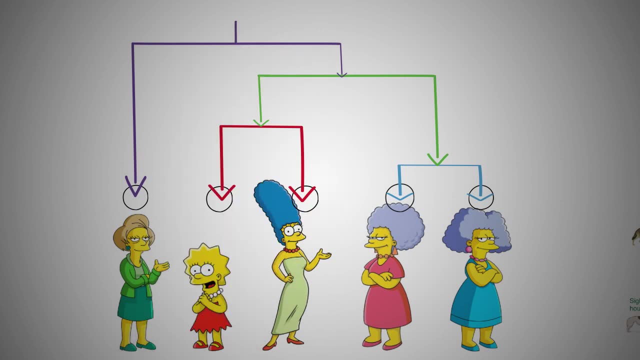 And you can see how long the process takes. Here you can see how long the branches is. So, looking at our dendogram, which shows how many clusters we have, as well as the order that they were clustered, We can then determine the significant clusters when we draw a threshold right about here. 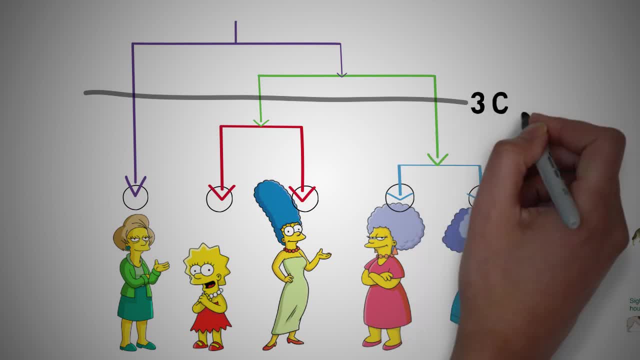 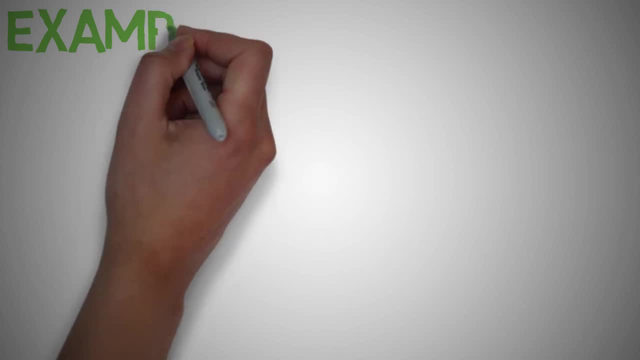 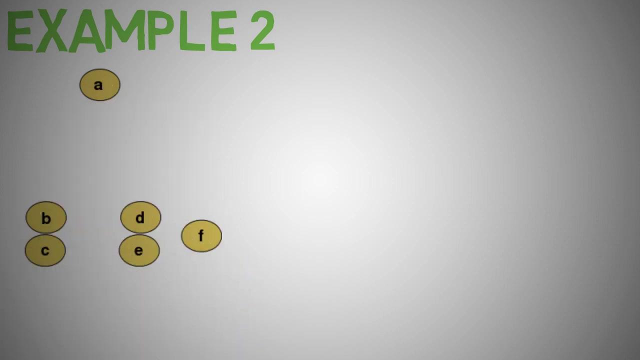 And we can obtain about 3 clusters based on hierarchical cluster analysis. Of course, we can adjust the threshold to suit our requirements. Ok, so let's apply what we've learnt from the previous example to a scatterplot of data. We have 6 points in our dataset, so that means that we have 6 clusters. 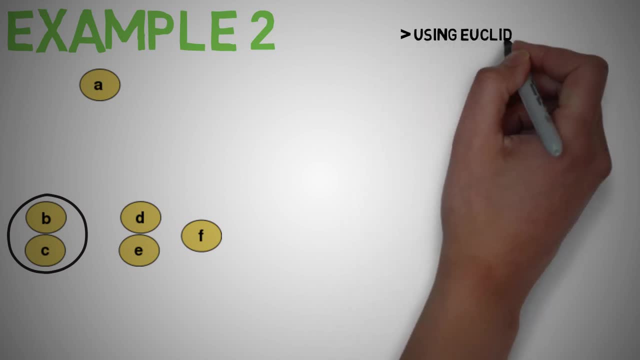 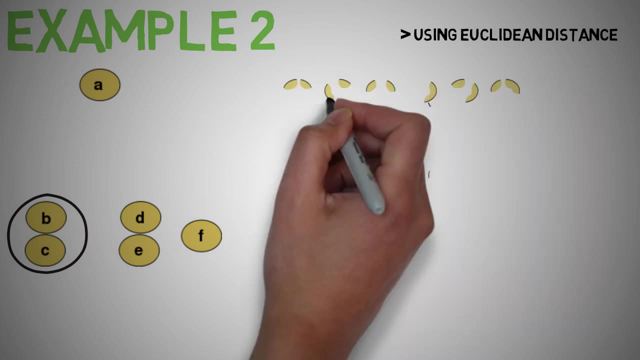 Let's start off with B and C and group them as they are close to each other, based on Euclidean distance, And this is our dissimilarity metric. You can use any other distance metric that you desire. Once we have B and C clustered, we can do the same for DE, which is more or less the 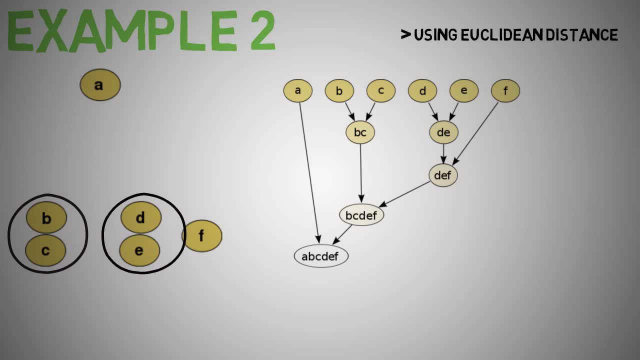 same distance apart as B and C. Next step: we join the clusters DE with F to form DEF- Notice how long the branch is from the F node- And then we can do the same but with node BC and DEF to form another one. And then finally we merge BCDEF with a much further cluster A. 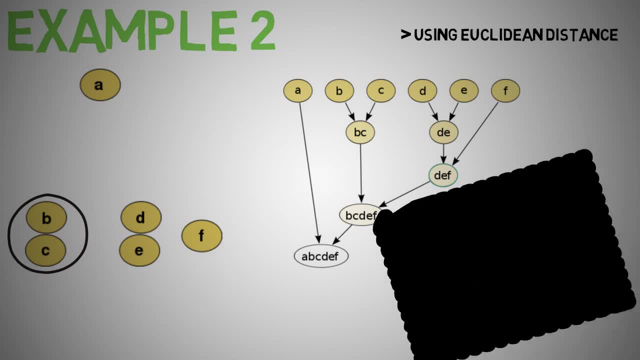 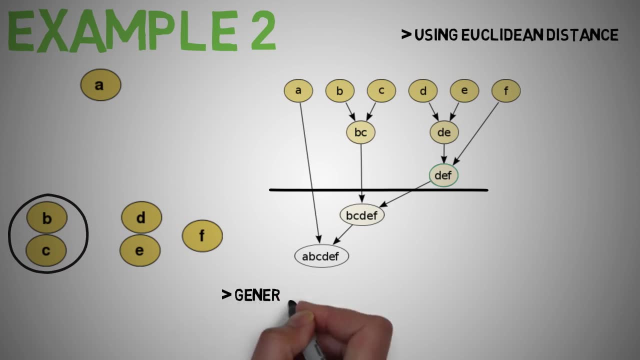 And now you can see from our dendrogram, we can choose our clusters as either 3 or 2 based on the threshold we place. Now, while there are many ways to find the optimal threshold, a general practice would be following For us to take the midpoint of the longest branch of our dendrogram and make that our 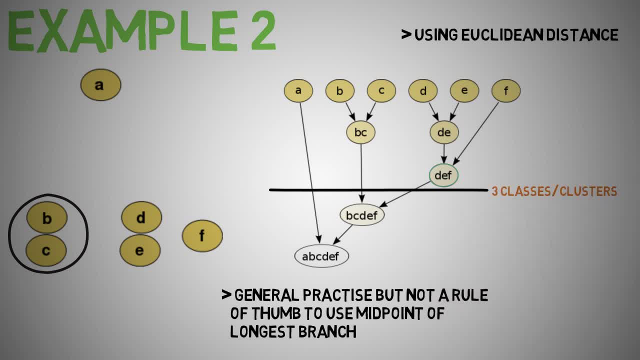 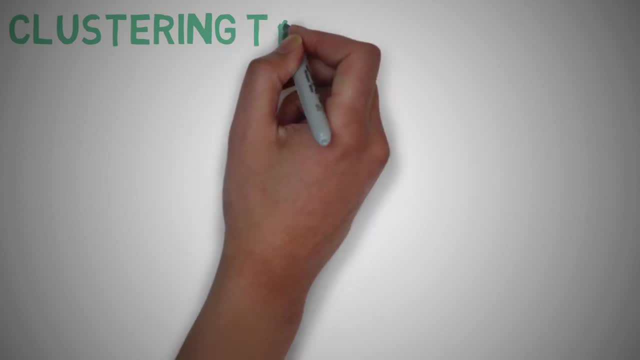 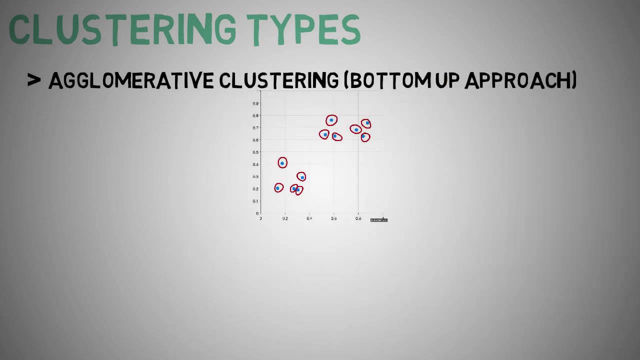 threshold, thus leading to 3 classes. I hope all this is making sense. on how hierarchical clustering works, So there are two main approaches with the HCA algorithm. They are agglomerative clustering, which is a bottom up approach that we performed in our previous two examples. 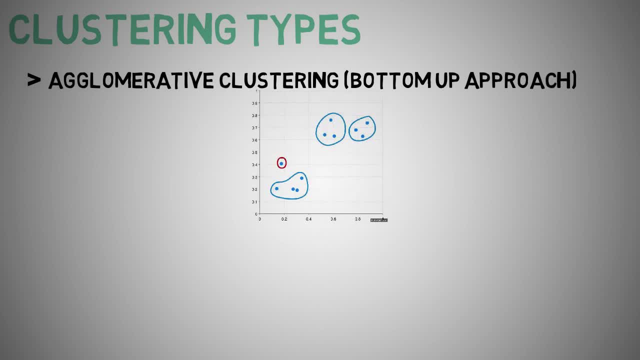 So, starting with each item as its own cluster, we find the best pair to merge into a new cluster. All clusters are fused together, And then there is the divisive clustering, which is a top down approach. It is less popular than the agglomerative method. 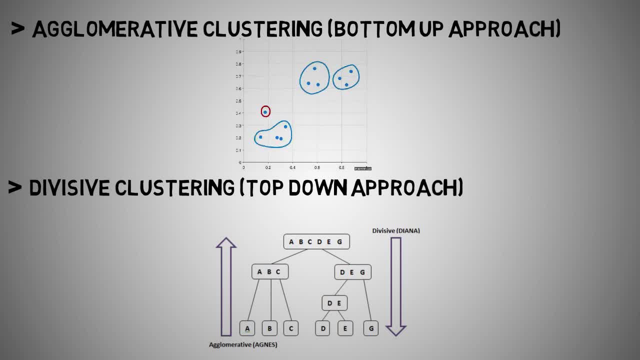 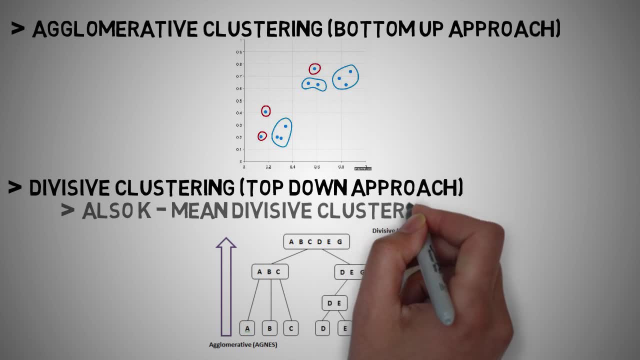 But with divisive. all observations start with one cluster and splits are performed recursively as one moves down the hierarchy. Now you get many variations of these approaches. You even get k-means- divisive clustering, But we won't go too deep into that yet. 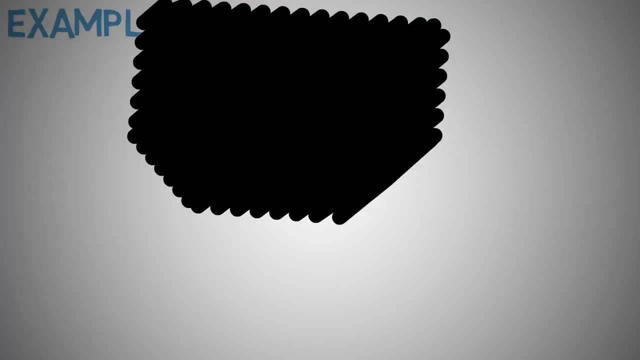 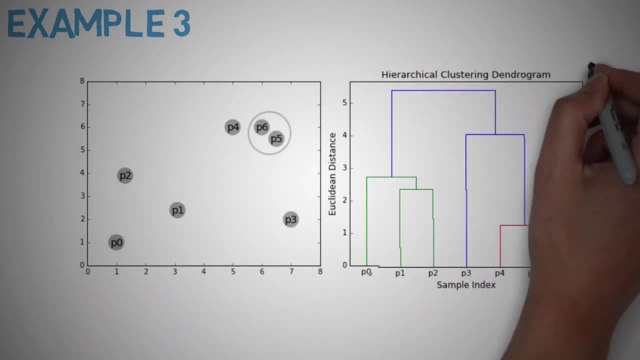 Let's take a look at one more example, Another one. So here is a dataset of 7 datapoints or clusters, in this case p0 to p6.. We start with the closest clusters, p6 and p5.. We use centroid linkage, which means that we use the Euclidean distance between the centroid. 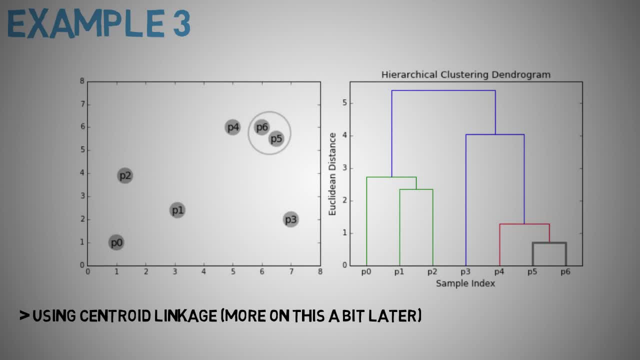 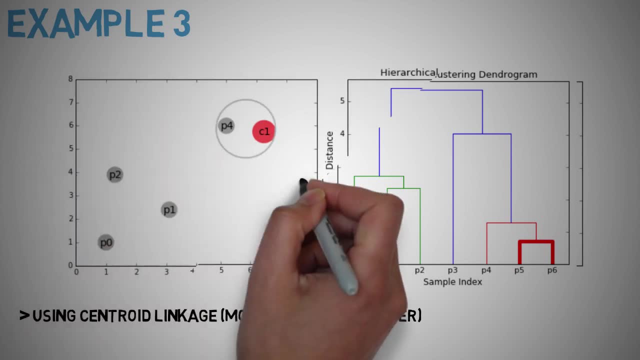 of the two clusters. We'll discuss other linkage methods later on in this video. So those two clusters become one cluster, co1.. So then we look for the next set of clusters that have the lowest Euclidean distance. In this case we have p4 and co1.. 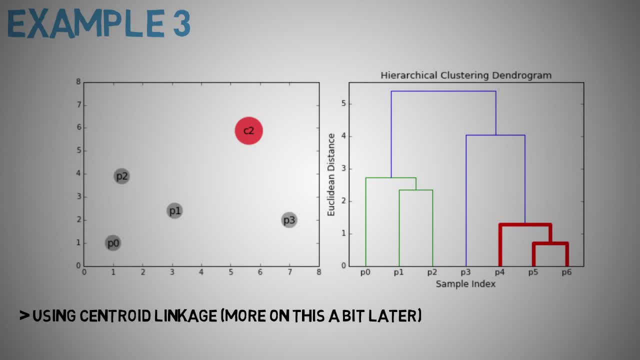 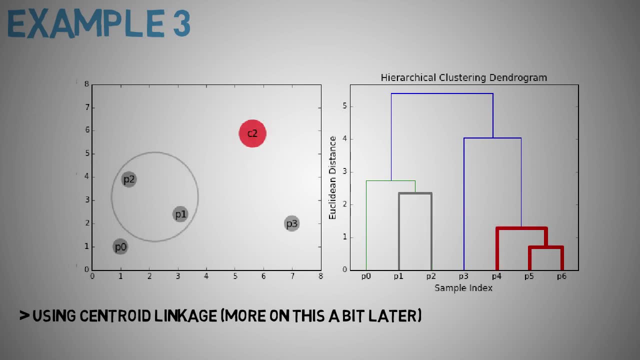 So here is a dataset of 7 datapoints or clusters. in this case, They join together to become c2. And this process is repeated for all the other clusters until there is only one cluster left. In the end, we can choose between 2 to 5 clusters, based on what the data represents. 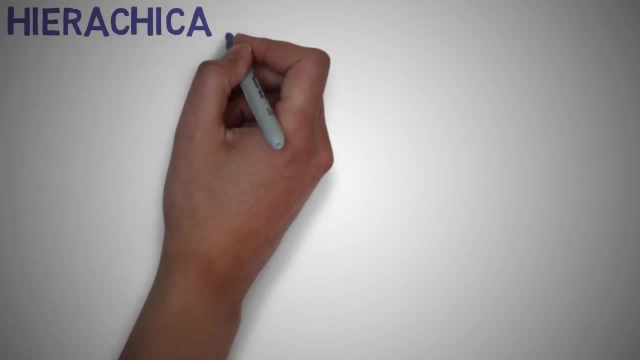 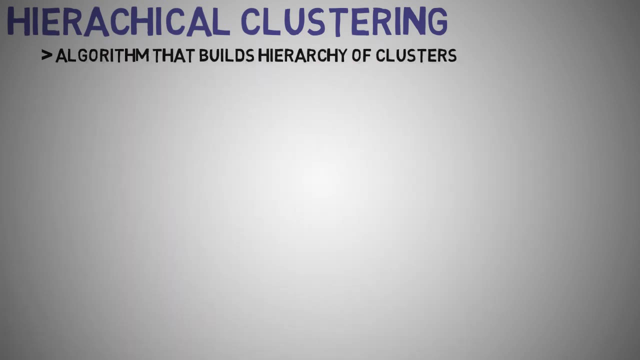 Easy right: Hierarchical clustering. Looking at the formal definition of hierarchical clustering, as the name suggests, is an algorithm that builds hierarchy of clusters. This algorithm starts with all the datapoints assigned to a cluster. This is the hierarchy of clusters. Then two nearest clusters are merged into the same cluster. 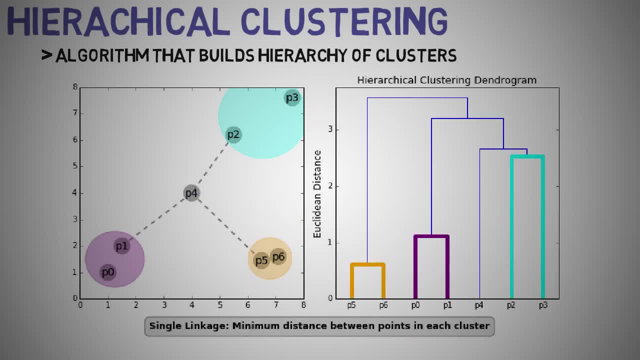 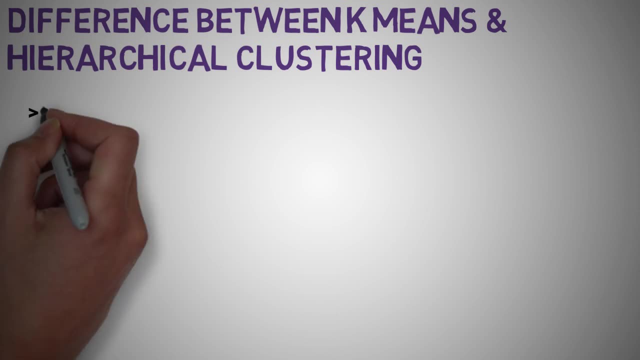 In the end, the algorithm terminates only when there is a single cluster left. The result of the hierarchical clustering can be shown using a dendrogram, as we've seen before, which can be thought of as a binary tree, Looking at the difference between k-means and hierarchical clustering. 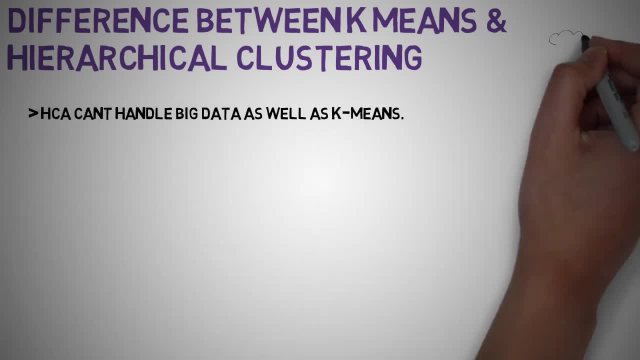 Hierarchical clustering can't handle big data well, but k-means clustering can. This is because the time complexity of k-means is very high. This is because the time complexity of k-means is very high. In fact, k-means is linear, while hierarchical clustering is quadratic. 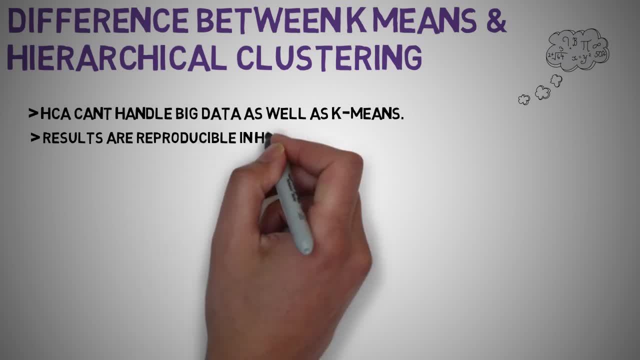 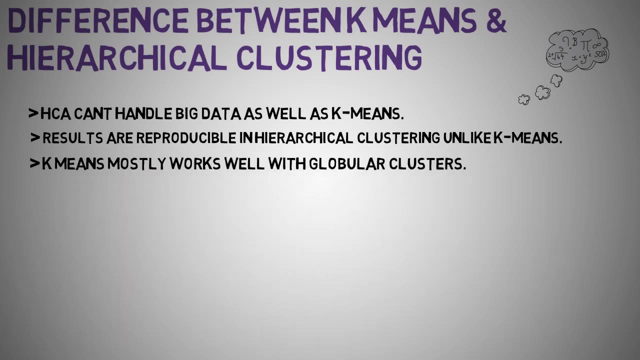 In k-means clustering. since we start with random choice of clusters, the results produced by running the algorithm multiple times might differ. while results are reproducible in hierarchical clustering, K-means is found to work well when the shape of the cluster is hyperspherical, like circle. 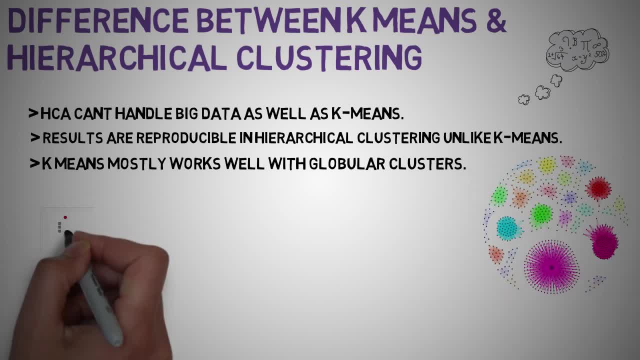 in 2D or sphere in 3D. k-means clustering requires prior knowledge of k, ie the problem of shadow resolve. • The number of clusters you want to divide your data into. However, with HTA you can stop at whatever number of clusters you find appropriate in. 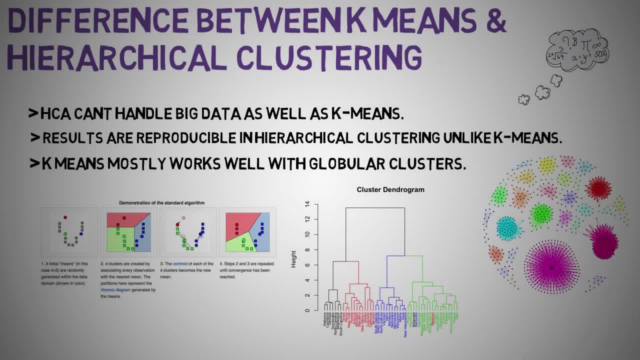 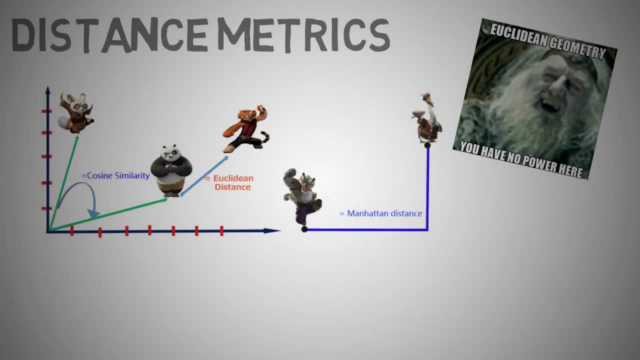 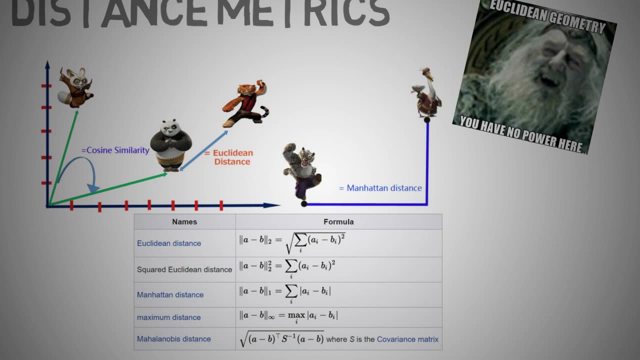 the hierarchical clustering by interpreting the dendrogram Distance Metrics. In a previous lecture of this series, we spoke about alternatives to the commonly used Euclidean distance, which are squared Euclidean distance, Manhattan or city block distance, maximum distance and Mahalanobis distance. 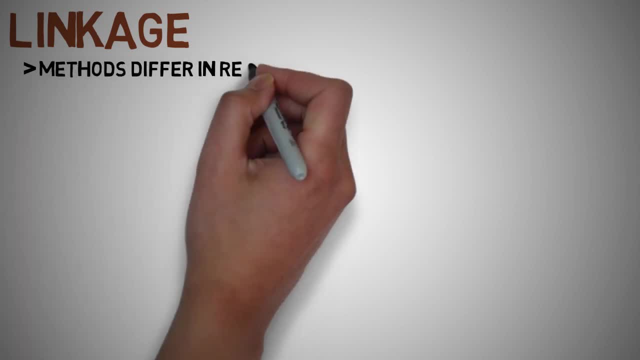 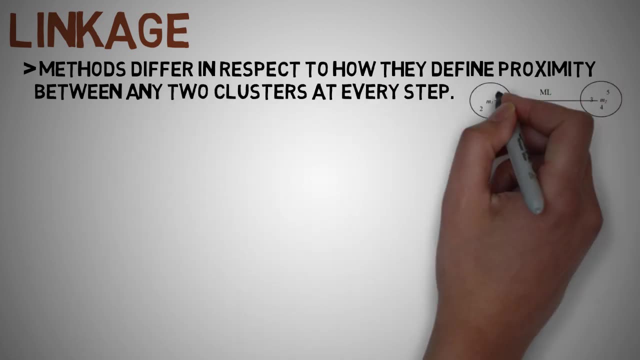 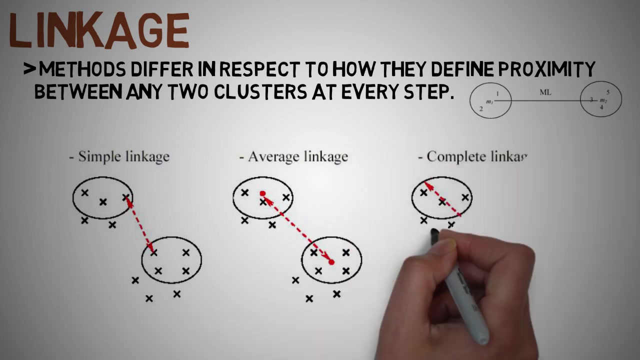 Linkage. So the methods differ in respect to how they define proximity between any two clusters at every step. In the previous examples we used the centroid of the clusters as our points to measure this similarity. So we have single linkage or nearest neighbour, where the proximity between two clusters is. 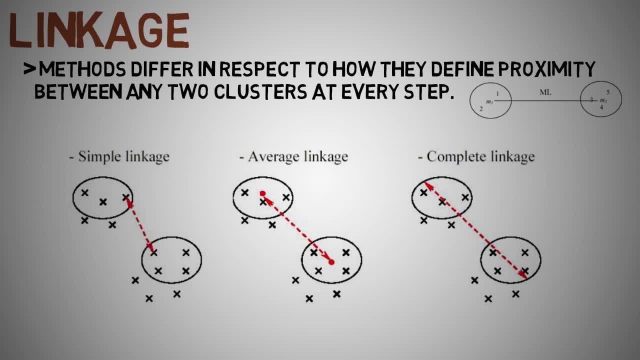 the proximity between the two closest objects. We have complete linkage, or the farthest neighbour, and proximity between two clusters is the proximity between their two most distant objects. And then we have the centroid method, where the proximity between two clusters is the proximity between their geomagnetic centroids, as we used in the previous examples. 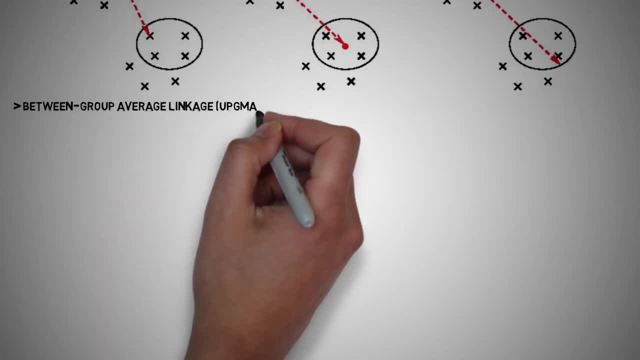 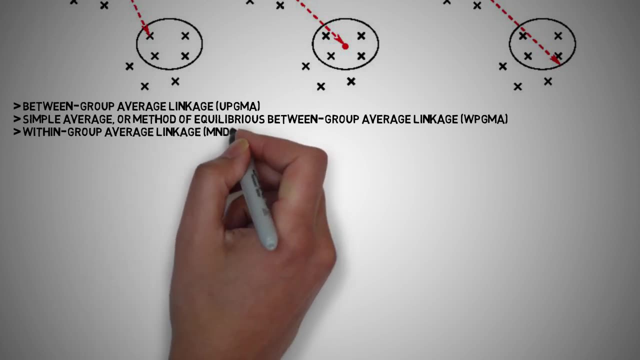 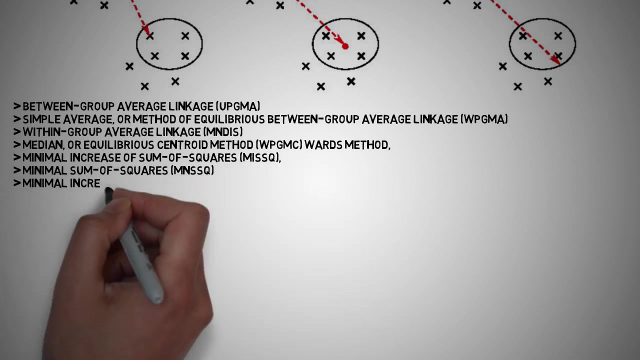 There are other linkage methods, such as between group average linkage, simple average or method equilibrium between group averages Within group average linkage Within group average linkage, Median or equilibrious centroid method, or also known as Ward's method. Minimal increase of sum of squares. 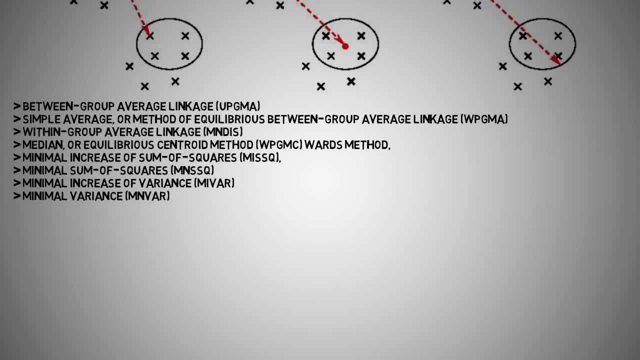 Minimal sum of squares, Minimal increase of variance And minimal variance. Shoo Sounds a lot. Why is this important? Well, as you can see from this image, if you select between either single linkage or complete linkage, for example, you end up with completely different sets of clusters. 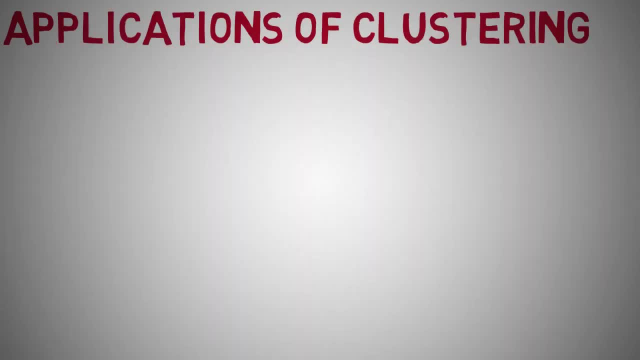 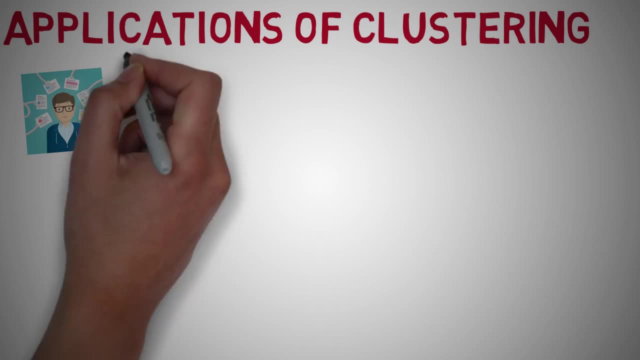 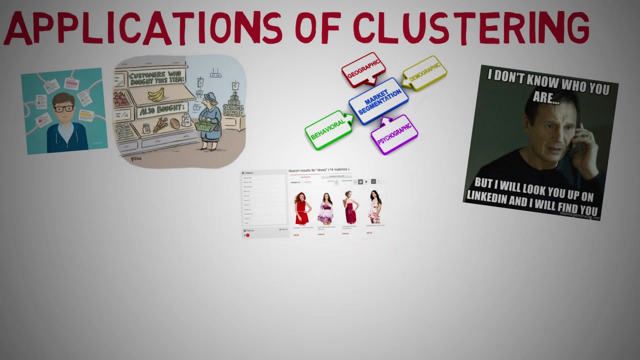 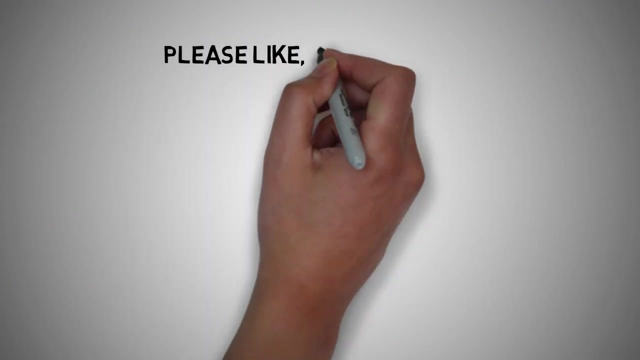 Applications of clustering. Clustering has a large number of applications spread across various domains. Some of the most popular applications of clustering are recommendation engines, market segmentation, social media analysis, search result grouping, medical imaging image segmentation and anomaly detection. So that is it from me.